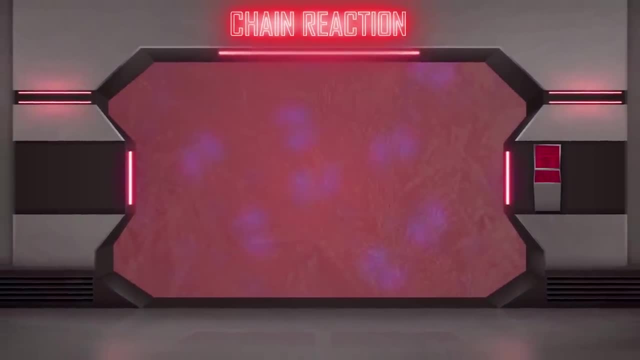 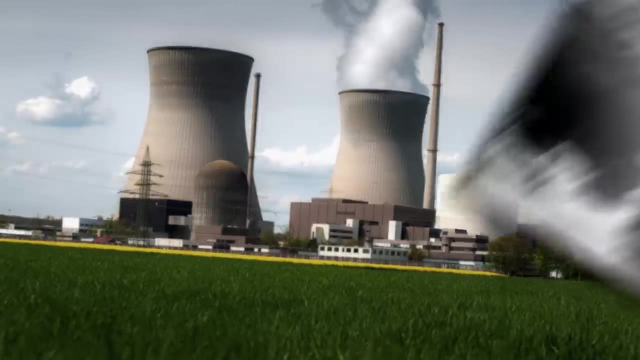 When a fissile is fissile. a fissile is a fissile, So if you have two or more neutrons each and you have a chain reaction. this reaction is an incredibly efficient way of releasing energy and is the reaction used in nuclear reactors as well as nuclear bombs. 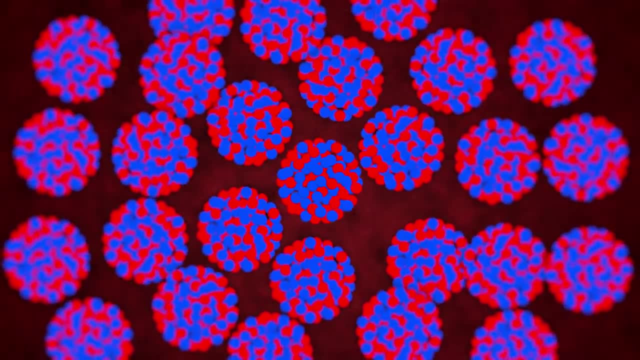 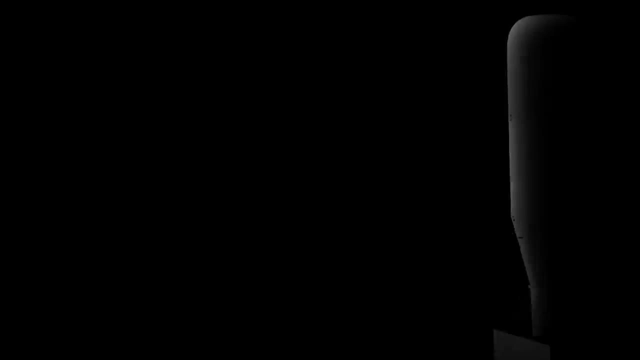 If we take enough nuclear fuel and pack it close enough together, we can force the fuel into supercriticality, which leads to an exponential growth of nuclear reaction and – you have a bomb – capable of devastation and atrocities. Our discoveries of the laws of nature: 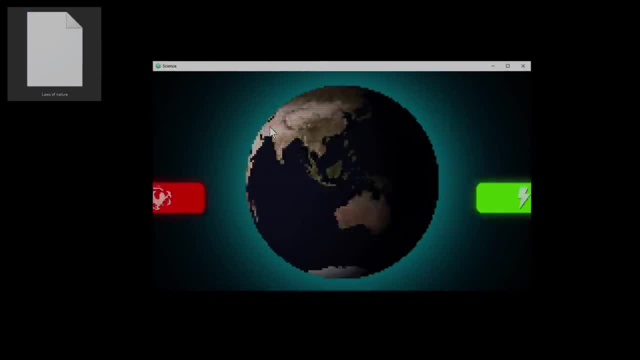 allow us to bend the screen a little bit, And this is what we're going to come up with now: bend the world to our will. What we choose to do with science is up to us. If we take the other path, we can choose to harness this highly efficient method of getting energy. 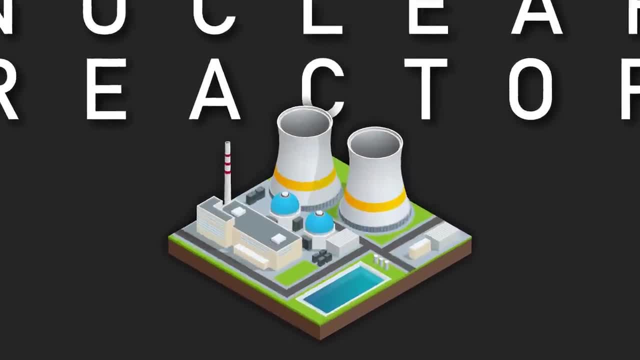 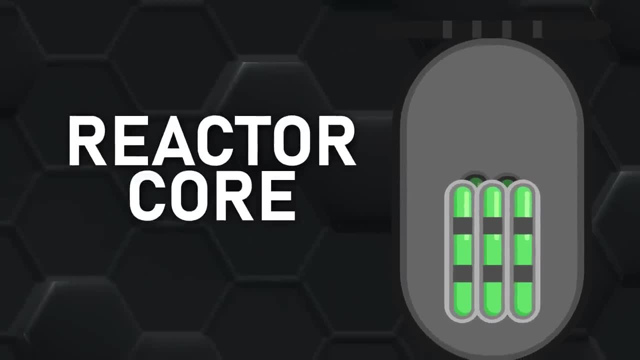 for good. Let's build a nuclear reactor. We'll take some nuclear fuel like uranium-235, put it inside a bunch of thin rods and put the rods inside a tank. This will be our reactor core. Inside the core we'll add a coolant, often water or molten salt, which will also serve. 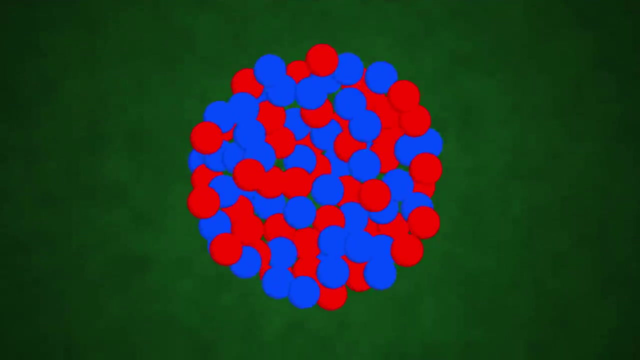 as a moderator. Why? For two reasons. Firstly, when neutrons are released from the nuclear chain reaction, they are released with an immense velocity. These fast neutrons, as they are appropriately called, would just bounce around the chamber and are very unlikely. 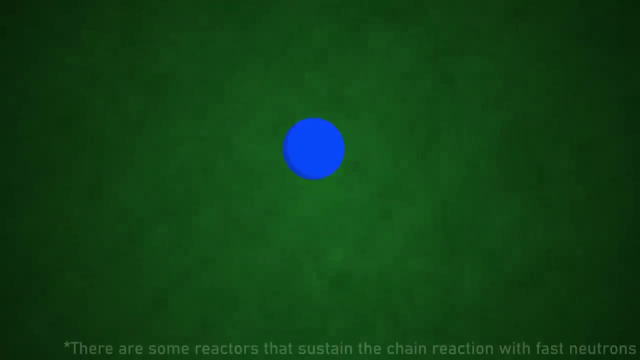 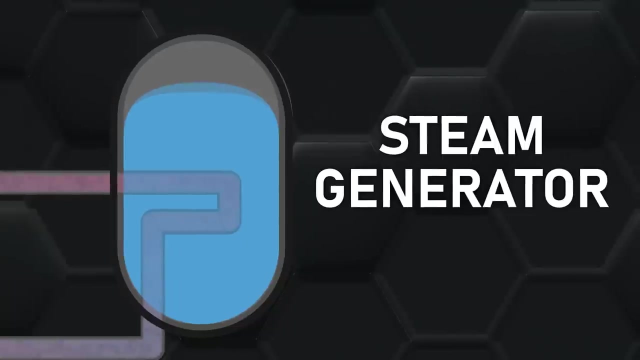 to really propagate the nuclear chain reaction. because of quantum mechanics, A moderator slows down these neutrons, leaving them as what are called thermal neutrons, which are way more likely to propagate the reaction. Secondly, this coolant allows us to circulate the heat outside of the core and into a steam generator. Here steam is generated, which 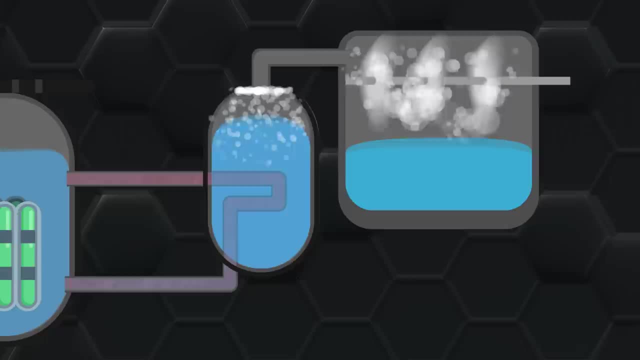 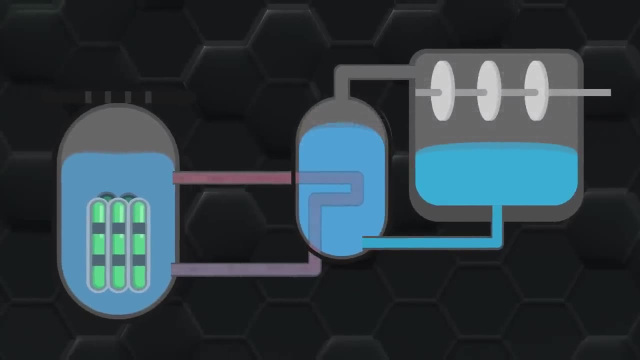 turns a turbine and creates electricity- Lots of it. The steam, now a lot colder, turns back into a liquid and is pumped back into the core again, where the whole process will repeat. Finally, we'll add some controlled rods to our reactor which are made of a neutron poison. These rods can be inserted or taken. 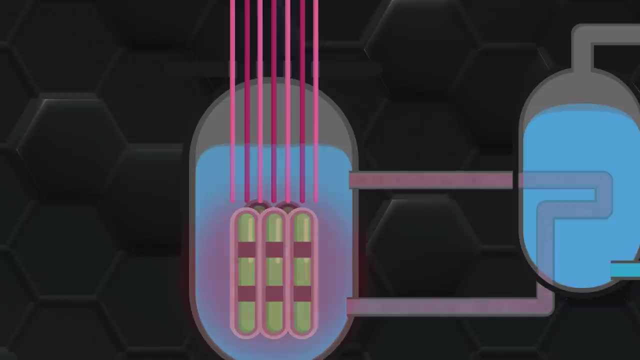 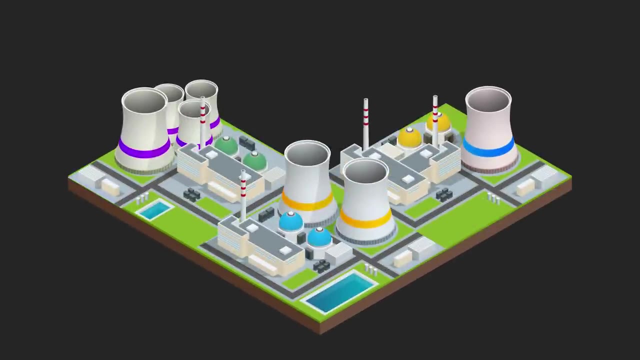 out of the core as necessary to ensure that the chain reaction happens at a steady rate. And that's how a nuclear reactor works. Kinda, there are a lot of different types of nuclear reactors, but in principle the concept is the same. Nuclear energy is quite a fascinating 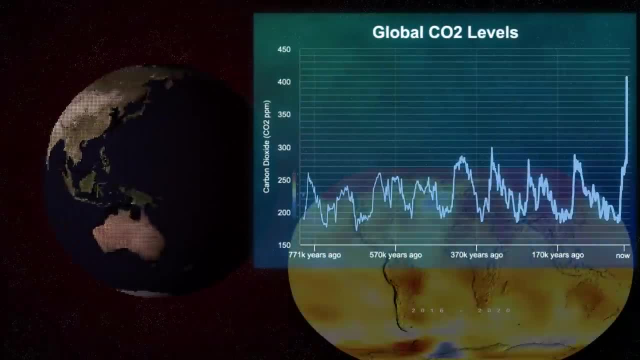 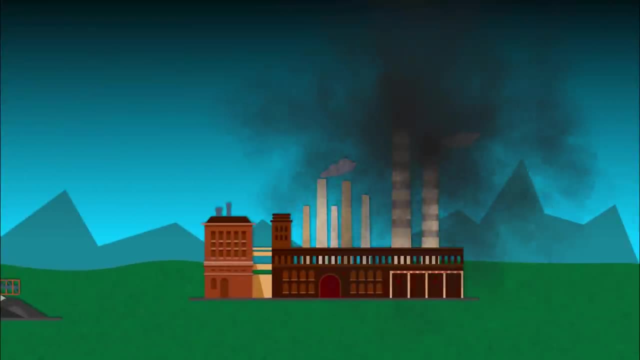 thing. Given the state of our rapidly changing climate, it would be wise of us to replace fossil fuels in favour of an energy source that doesn't entail removing carbon from the ground and pumping it into our atmosphere. Renewables like wind, solar or hydroelectricity would 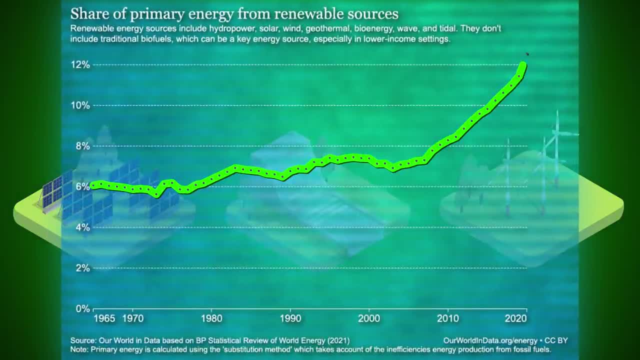 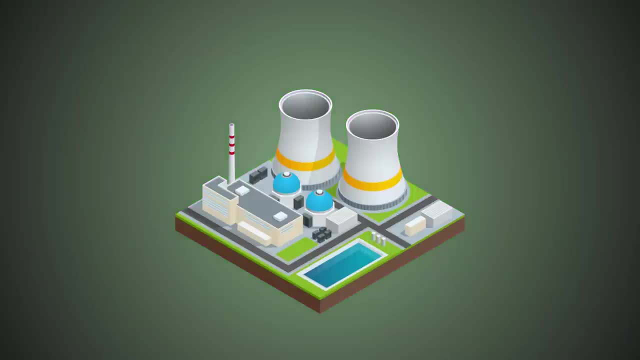 be the obvious long-term choice, but we're quite slow to adopt those, aren't we? Nuclear energy could be a transitional source of energy while we build more renewables. Nuclear energy is obviously not perfect, though, with the nuclear waste that is generated from nuclear. 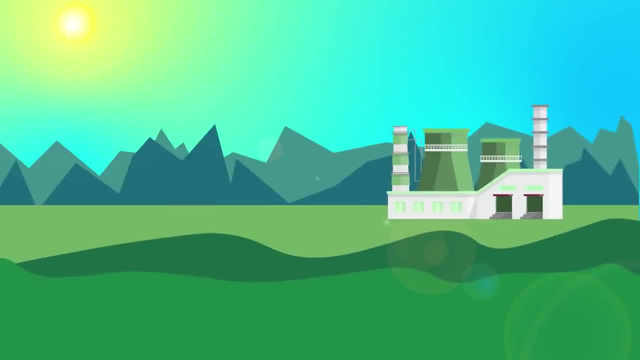 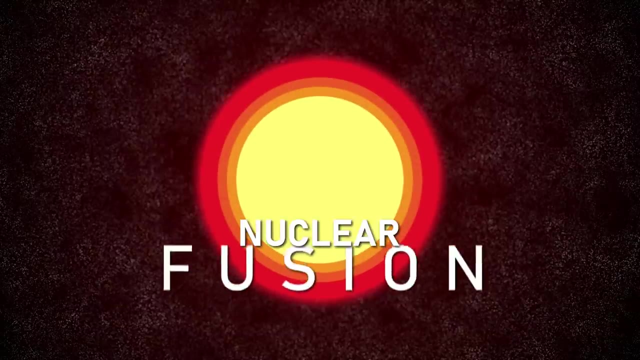 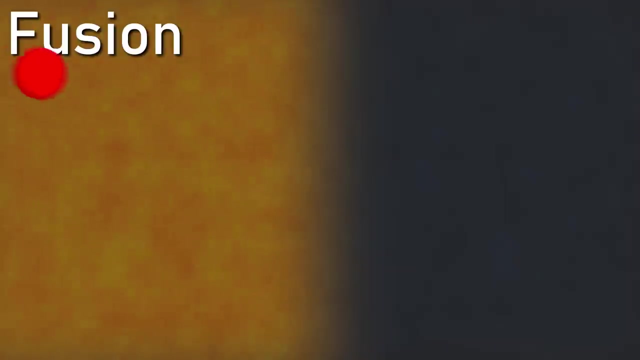 reactors. If only there was another reaction that could produce a ton of clean energy. That would be great, wouldn't it? This is a working nuclear fusion reactor. Let's go inside it. In here, the core of the star is where the magic happens with the fusion. Nuclear fusion, oppositely to 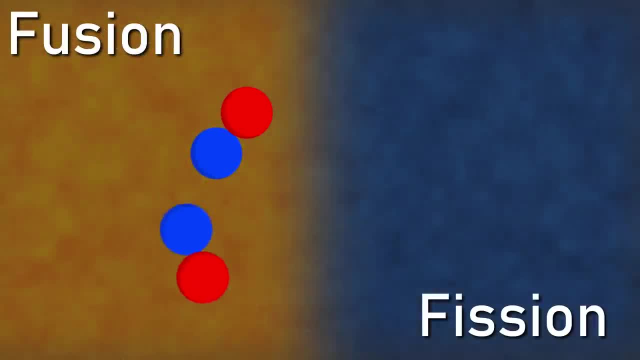 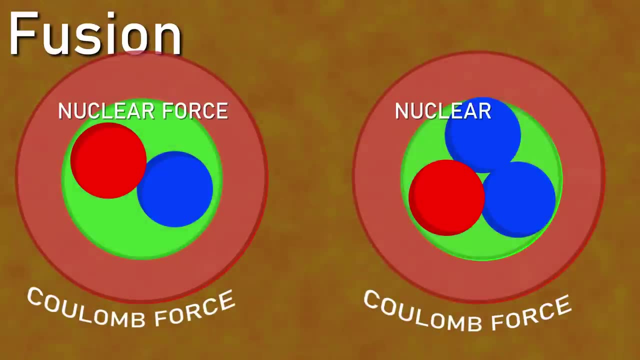 nuclear fission is when two or more nuclei combine. Interestingly enough, this process also releases a ton of energy because of the two opposing forces, that are the coulomb force and the nuclear force. Protons are positively charged, which means they repel each other. 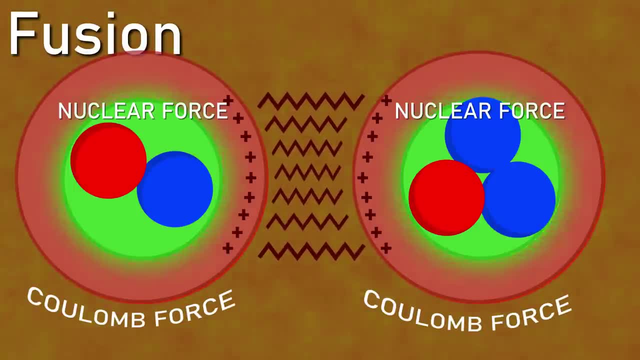 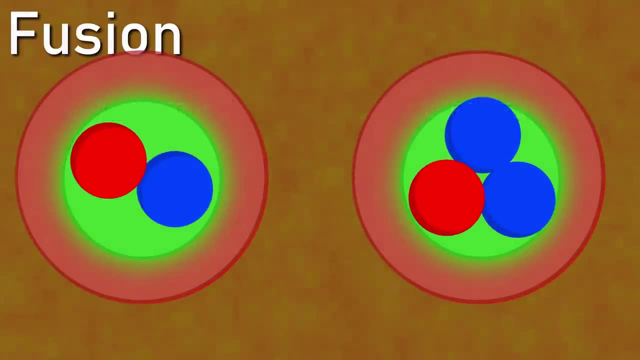 This is the coulomb force. There is another, stronger force though, the nuclear force, which allows the protons to combine. This force, however, is only strong at very small distances. For two nuclei to combine, there is a huge energy barrier that must be overcome. 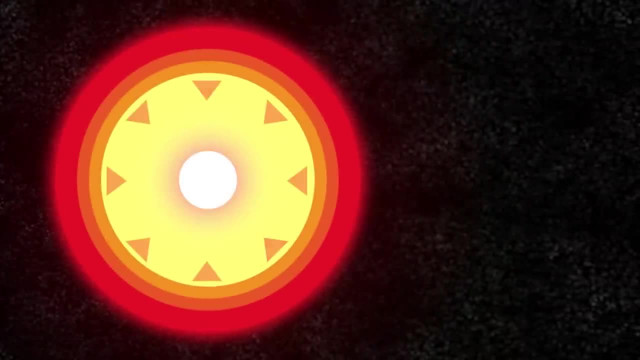 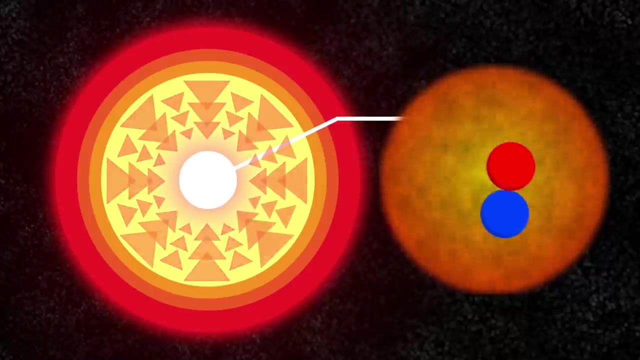 These conditions are met inside the core of the sun, as it's so huge that the pressure and heat in the core squeeze the nuclei together. When two small nuclei fuse, a ton of energy is released. It's this energy that powers the sun, and wouldn't it be great if we could. 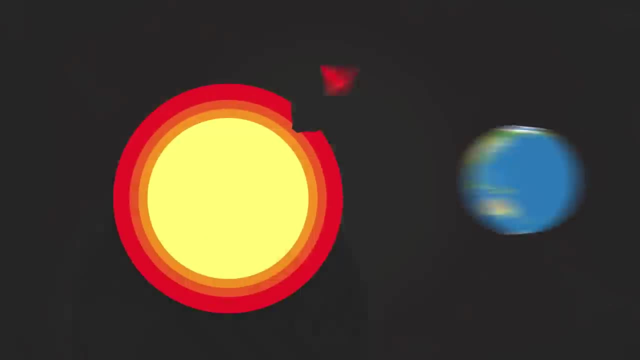 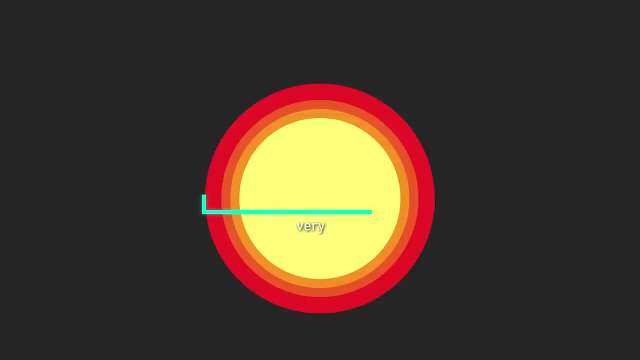 do the same here here on Earth. Slight problem though: we can't just take a piece of the sun with us back to Earth and use that for energy. The fusion in the sun works precisely because the sun is so huge. so if we want to use fusion energy here on Earth, we're going to have to find 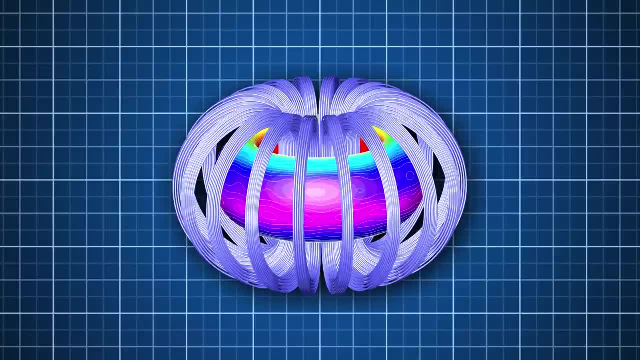 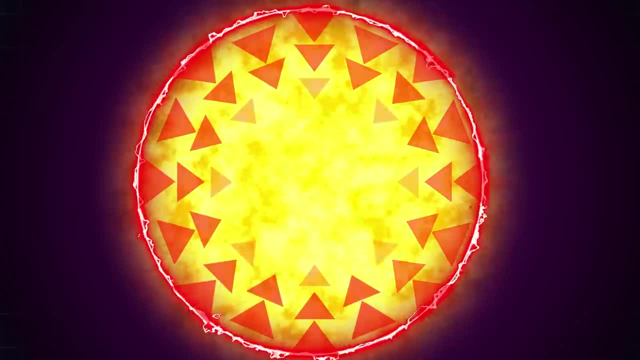 different ways to create the conditions necessary for fusion to happen. As it turns out, that isn't all that difficult. Doing a little fusion is no problem, but if we want to create the proper reactions to generate a remarkable amount of energy, we're going to need to. 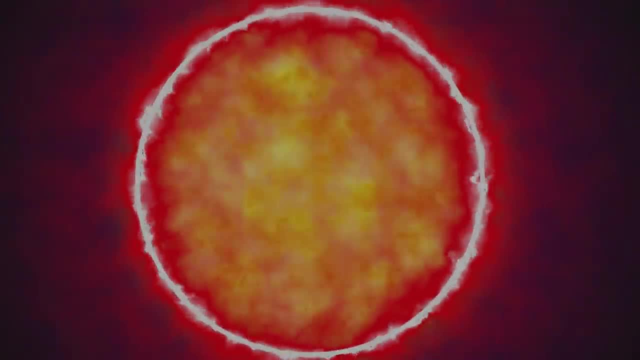 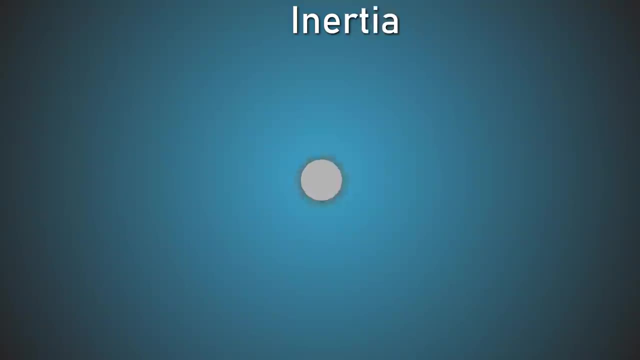 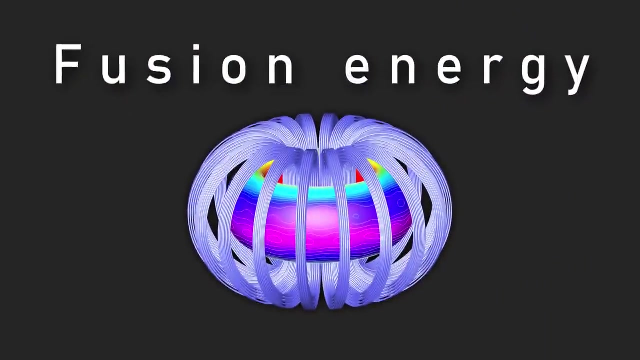 be creative. Currently, the two leading branches in the quest for fusion energy are magnetic confinement, which utilises magnetic fields to create the proper conditions for plasma, and inertial confinement, which uses incredibly strong lasers to compress and heat fuel pellets. The biggest issue with fusion energy today as an energy source isn't the fusion reaction.